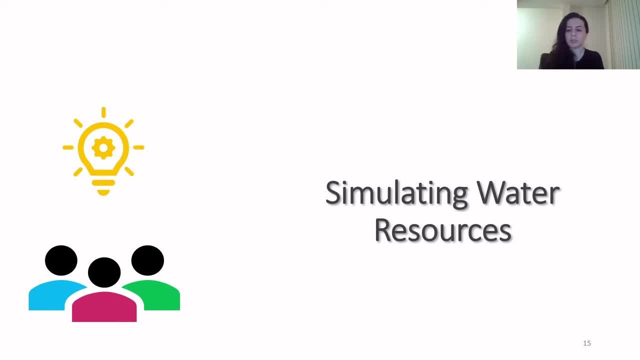 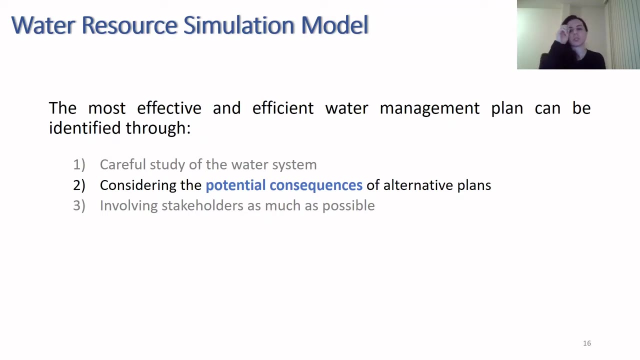 we can simulate water resources and how this simulation can help us manage our water resources in a better way. Recalling from the first part of this lecture, finding the most effective and efficient water management plan can be achieved through some considerations, and one of them was: 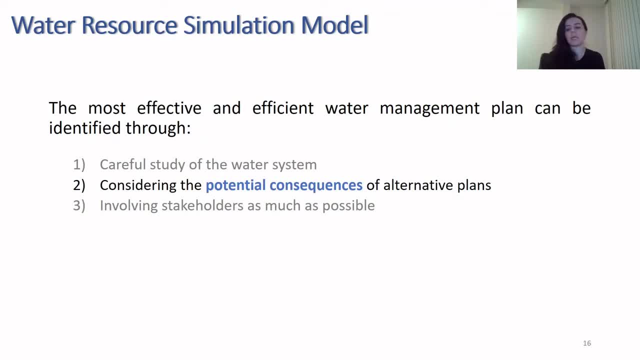 considering the potential consequences of alternative water management strategies and plans, So we can understand and estimate these consequences, using a simulation model, in a way that tells us, or predicts for us, how a change in the system can affect the water system of the river basin. So to do this, we can define scenarios as 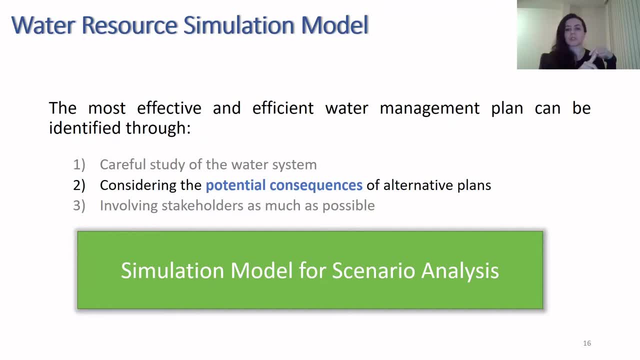 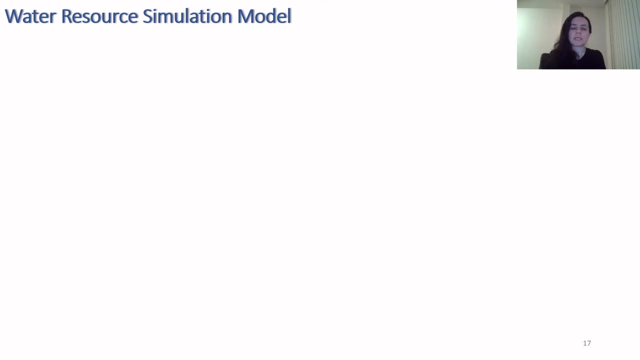 water management strategies or other external drivers like climate change or socio-economic developments that make a change to the water system, and then simulate the system to estimate or to evaluate the impacts of those changes on the water universities. Now let's see how we can simulate water resource system. 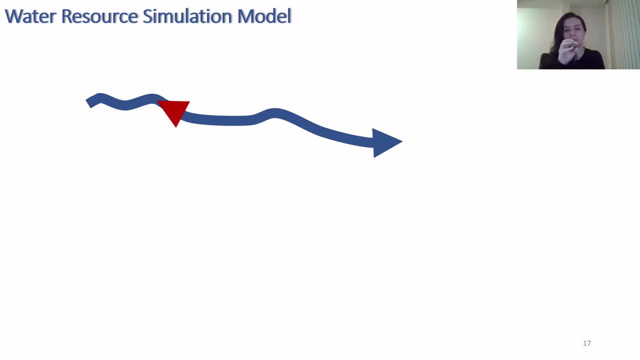 Here is a simple short river ridge with a reservoir on it and we are going to try to make a simulation model for this small water system. So we have, in each time step the T, we have the inflow into the reservoir and the flow in the river downstream the reservoir. 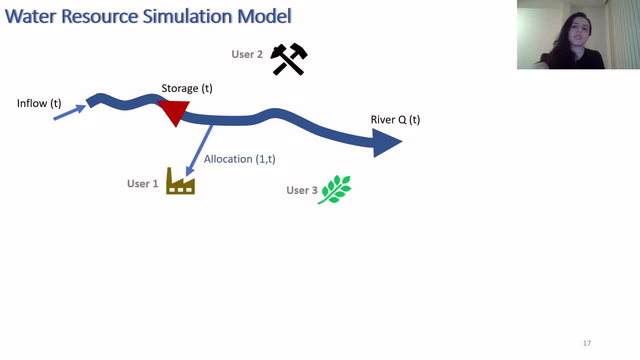 Also imagine that we have three users receiving water from this system. So allocation 1T is the amount of water that this reservoir releases for the user number one at time, step T. And now assume that we know the priorities of these users in receiving water. 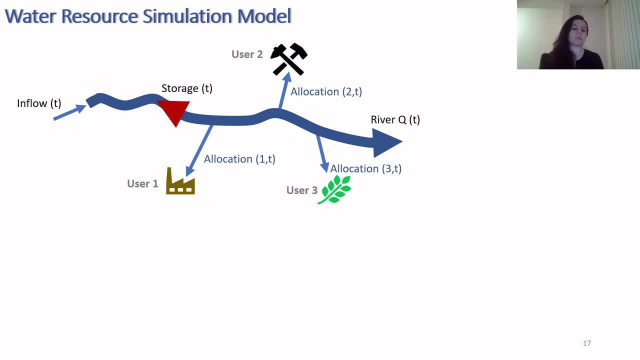 So we know that which user should receive water first, And this is called the priority system here. To define this priority system in our model here we use a penalty system, meaning that we assign penalty values to each of these users corresponding to the amount to the priority of these users. 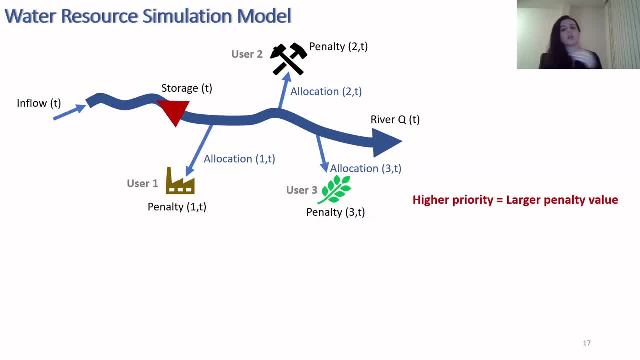 So the higher the priority of the user, the larger the amount, the value of that penalty. And then the model tries to allocate water to different users in a way that minimizes the total penalty for all these three users. So you can see that the model is based on a simple optimization problem. 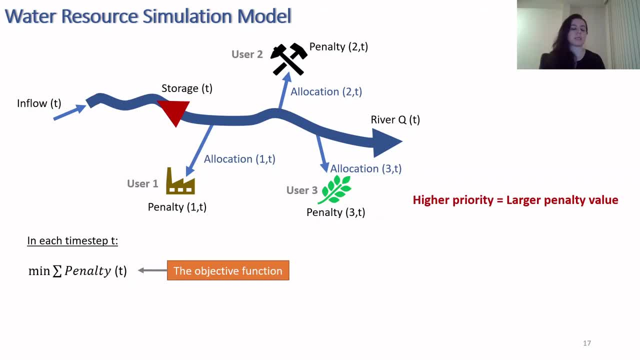 with an objective function, that is, minimizing the total penalty among different users here. But in each time step we need to conserve the mass balance of water which is here. the storage of the reservoir in each time step should equal to the storage of the reservoir in the previous step. 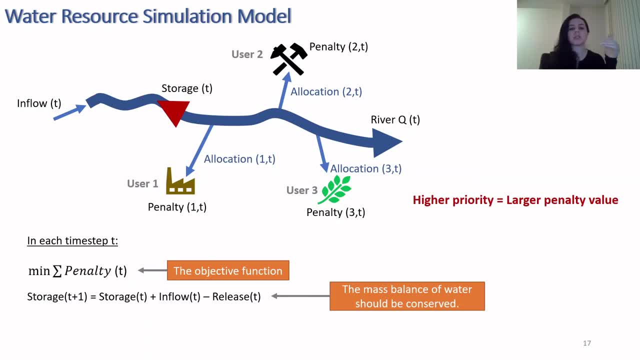 plus the inflow in that time step, minus the release from the reservoir. And how do we define release here? The release includes all the allocations to different users plus the amount of flow that we want to see In the river downstream the reservoir. This flow can be used for other users downstream, further downstream. 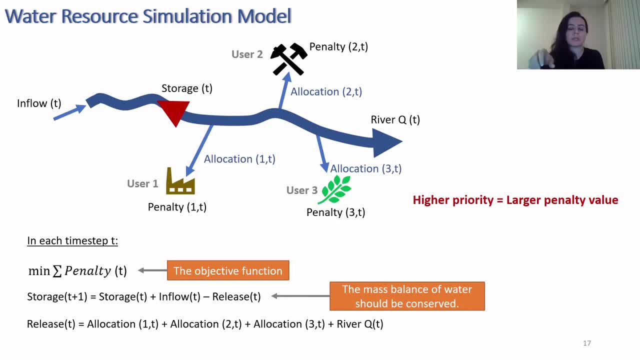 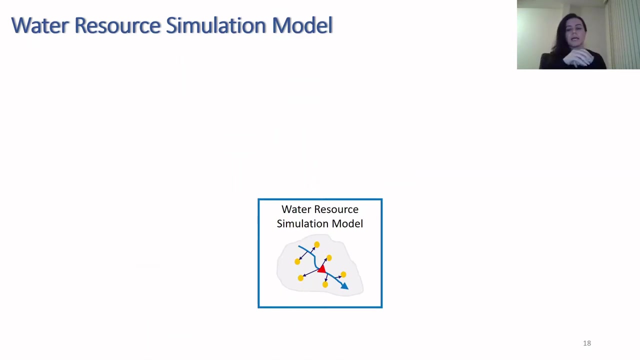 or can be considered as the environmental water requirement in the river. Now here we can say that so far we made the mathematical model to simulate this river ridge. But now if we want to look at the structure of the model and what are the requirements to develop this model, 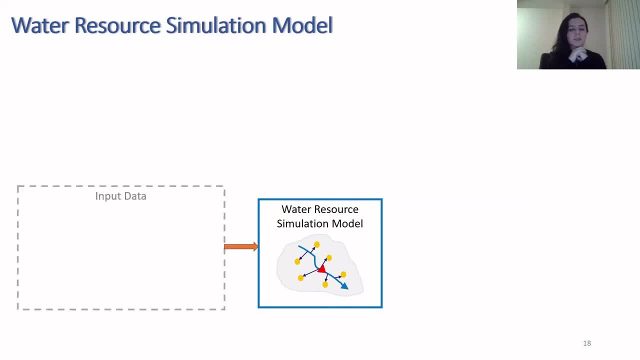 we can see that we need a set of input data And, as I explained, we need inflow time series for each river tributary that we are or river ridge that we are including in our model. Also, we need water demand time series. 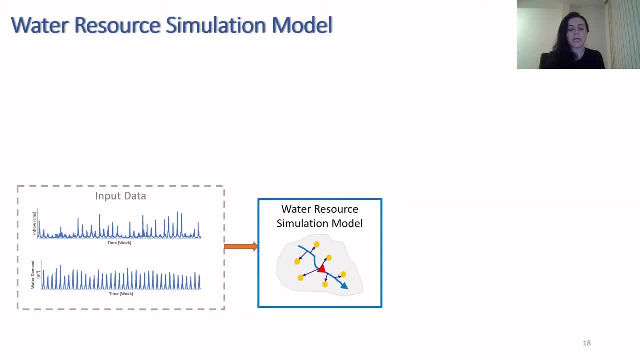 for each user that we consider in our model. So this time series shows the amount of water required by each user at each time step. Apart from input data, we need system configurations to be defined for our river basin or the river system that we want to simulate here. 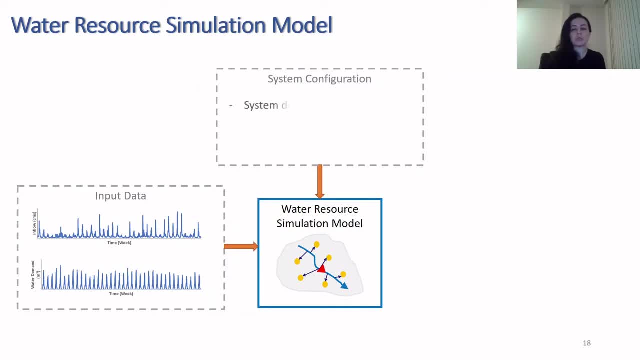 And this system configuration includes system designs, meaning the designing characteristics of different infrastructures that are included in our modeling exercise, For example reservoirs or diversion systems, And these designing characteristics include, for example, the capacity of these infrastructures. Also, we need to define reservoir operating policy. 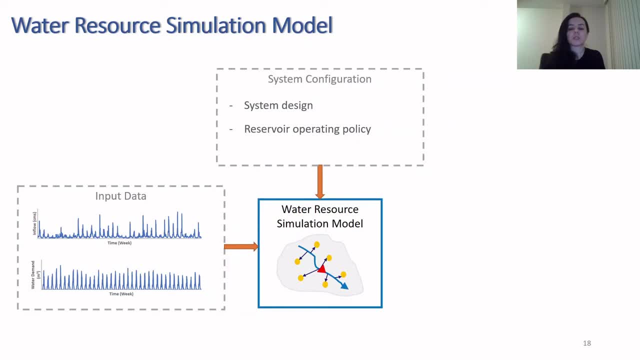 And this policy shows that how much water should be released in each time step, based on the storage of the reservoir. Also, we need to define reservoir allocation policy, meaning that from the amount of water that is released from the reservoir, how much should go to each reservoir. 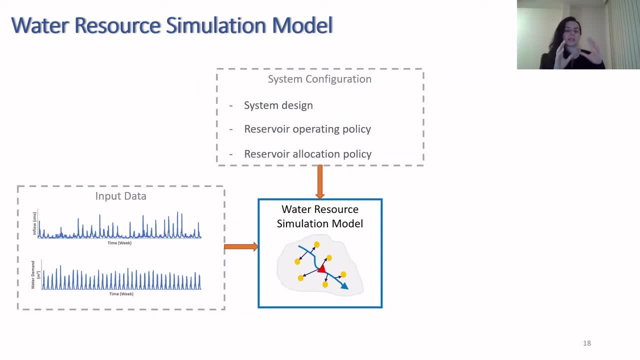 for each user. When we define these system configurations and we enter the input data into the model, then we can run the model and the model generates some outputs. These outputs can be in the form of water supply and shortage for different users, For example, irrigation and non-irrigation users. 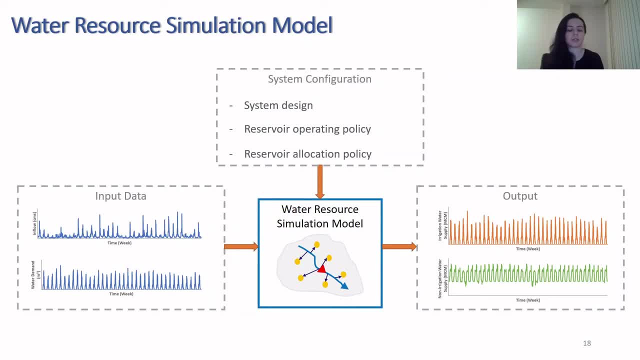 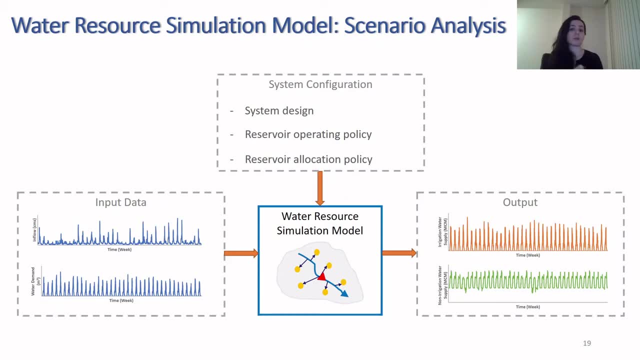 Now how we can use this modeling structure for scenario analysis. Well, depending on the type of scenario that we are defining here, each scenario may change input, data or system configuration. For example, if we have a climate change scenario, the inflow time series should be changed. 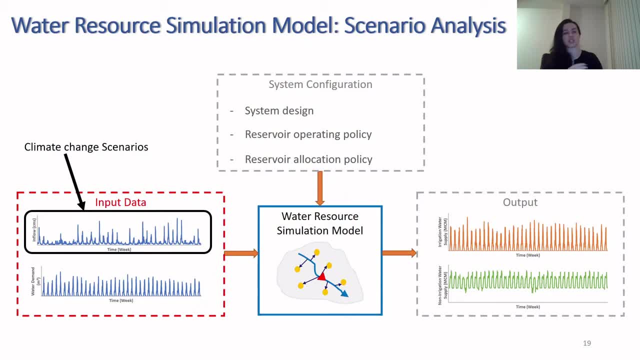 according to that scenario. because climate change scenarios basically change temperature and precipitation and other climatic variables that directly affect the inflow in river reaches, So we need to replace the inflow time series under the status quo with the new time series under the climate change scenario. 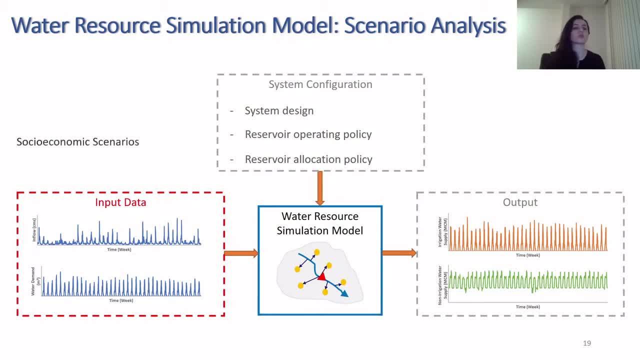 that we want to explore. Also, socioeconomic scenarios change the input data And that is because these scenarios change the demand for water. For example, consider a population growth scenario or an irrigation expansion scenario. These scenarios change the demand for water at municipal or agricultural sectors respectively. 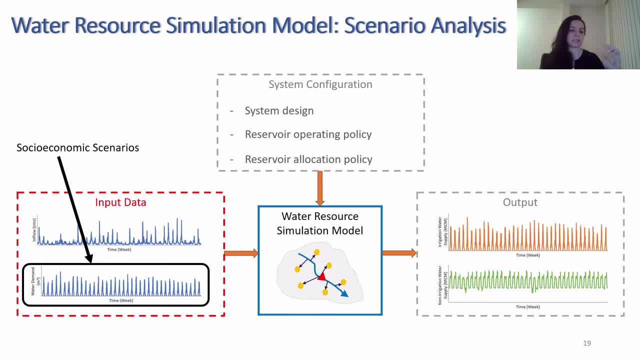 Then we need to replace the demand time series in the model with the new demand time series under the socioeconomic scenario that we want to study. There are other scenarios that change and alter the system configurations, And these scenarios include infrastructure scenarios that change the system design. 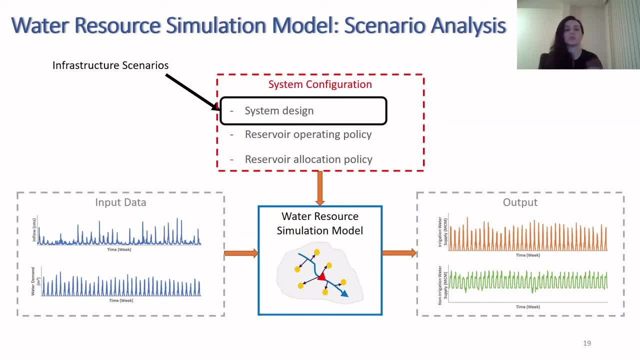 Imagine that we want to construct a new dam or a new reservoir, Or we want to change the capacity of a diversion channel in the system. So we need to change the designing characteristics of the system according to the characteristics that we consider under that specific scenario. 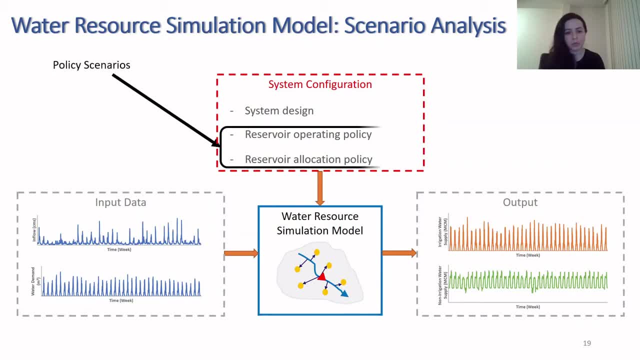 Also other scenarios, like policy scenarios, change the system configurations. For example, a policy scenario may change a reservoir operating policy or a reservoir allocation policy. For example, if we want to reallocate water among different sectors in a region, we need to change the allocation policy. 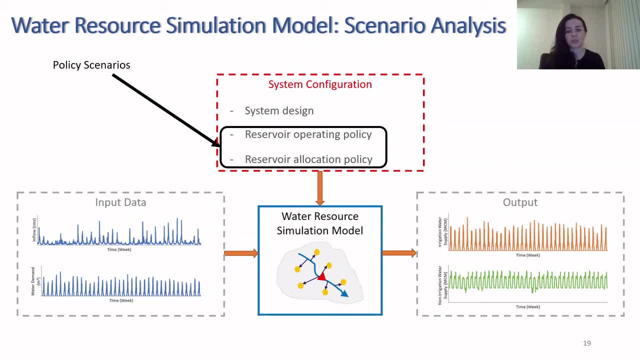 that we already have in the water resource simulation model. And when we replace all these changes and when we update the model with the scenario analysis purpose, then we can run the model and then we can see the outputs of the model. And by comparing these outputs, 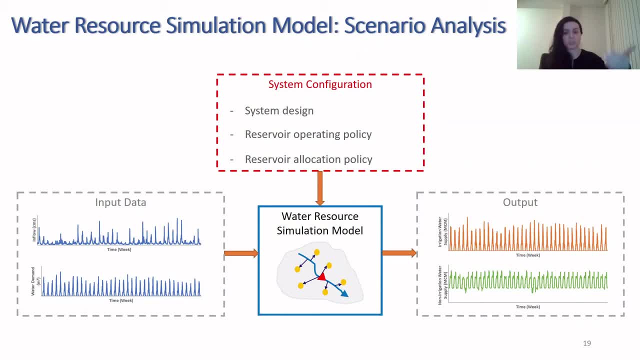 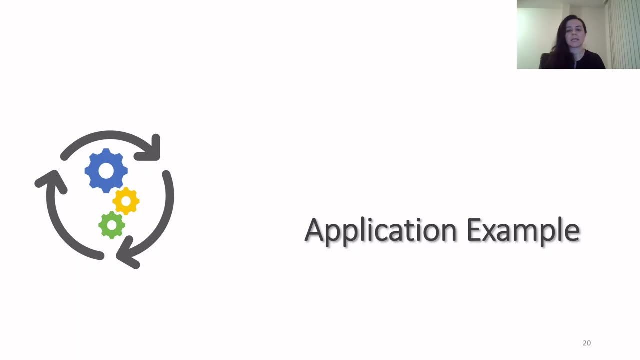 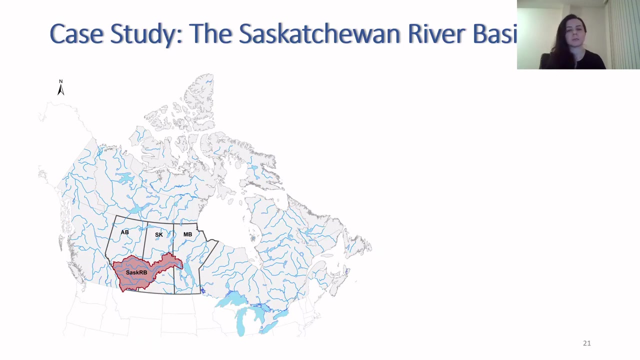 with the outputs under the status quo before the change, we can see how this change affects the system and the performance of the system. Now, to better understand how we can use these models, let's take a look at an application example. This example is a study conducted. 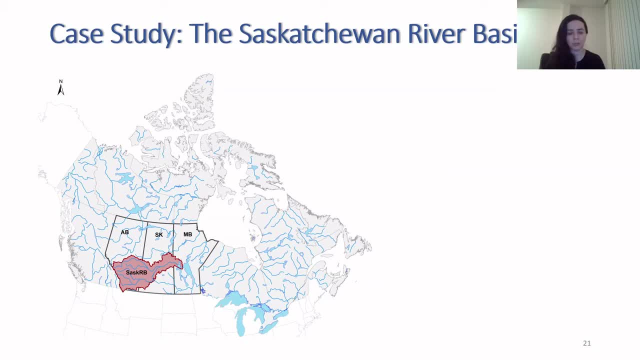 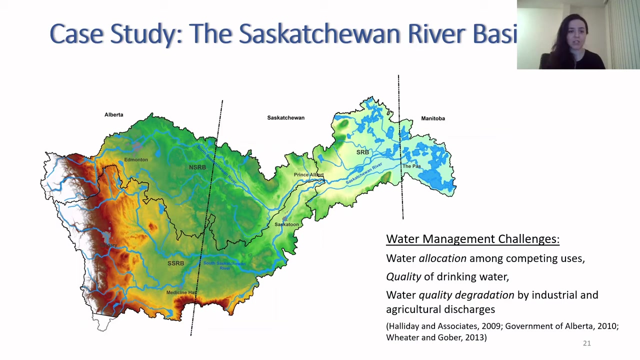 in the Saskatchewan River Basin in Canada. This river basin encompasses three Canadian prairie provinces and is a large river basin facing a number of water quality and water quantity challenges. Just to give you an idea about the challenges- water management challenges- that this river basin is facing: 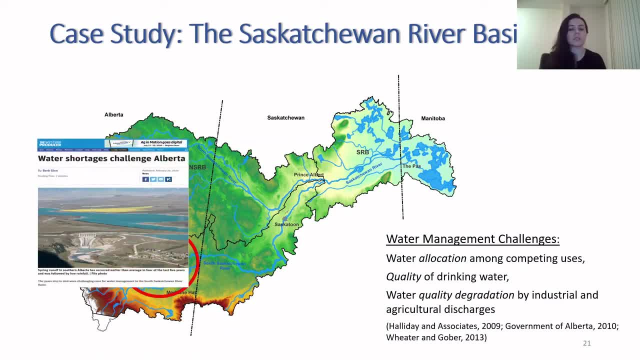 I can mention water over-allocating challenges in upstream regions. that prevents water authorities from issuing new licenses for new usages in those areas. Also, in downstream regions, people and mostly indigenous communities have been facing several water quality issues And still there is need. 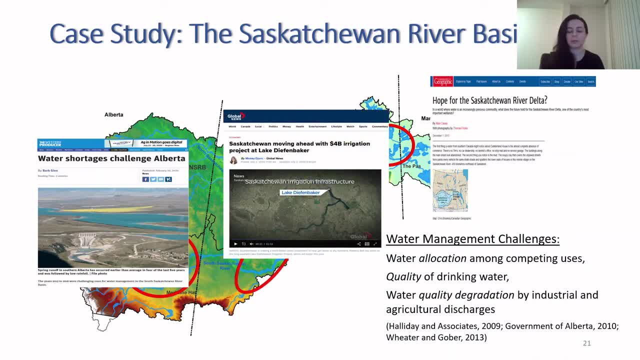 for more development in some other parts of this river basin, for example, the need for irrigation expansion in the province of Saskatchewan. So in this example, we developed a water resource simulation model for this river basin and we used it to see the impacts of irrigation expansion. 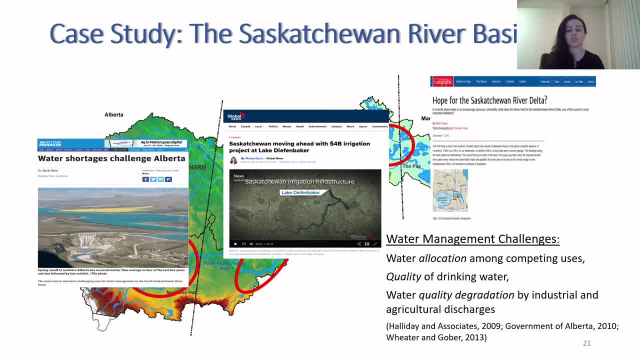 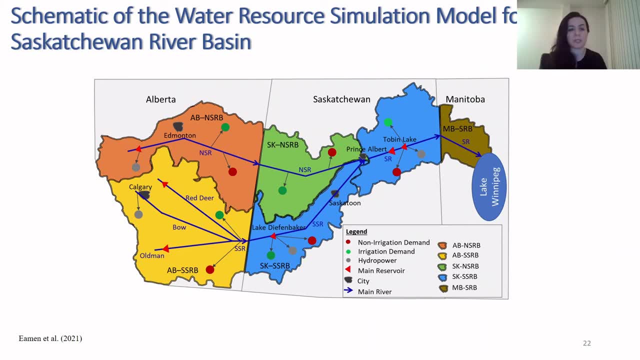 on the performance of water system in this river basin. Here is the schematic of the water resource simulation model for the Saskatchewan River Basin, And the sub-model and the part of this model that I'm going to use in this example and show the results is developed for this blue part. 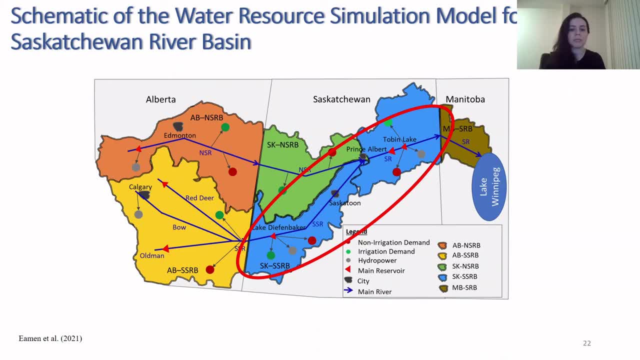 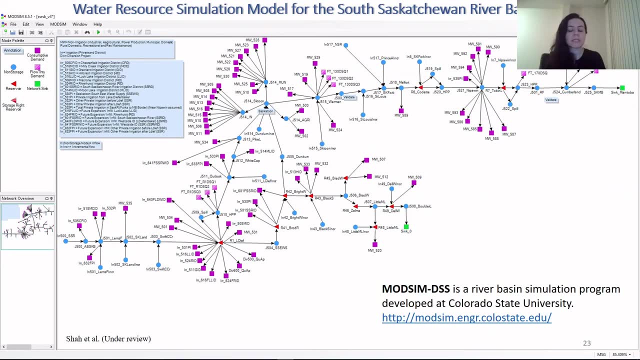 known as South Saskatchewan River Basin, And here's a snapshot of the model developed for this part. This model is developed in MOTSIM DSS platform, which is a river basin simulation program developed at Colorado State University. This is a node link network where nodes represent water resource or demand sites. 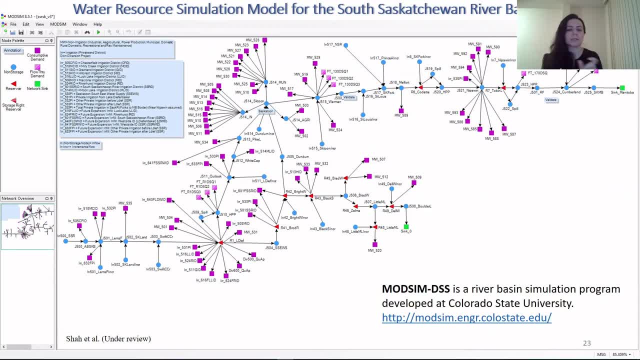 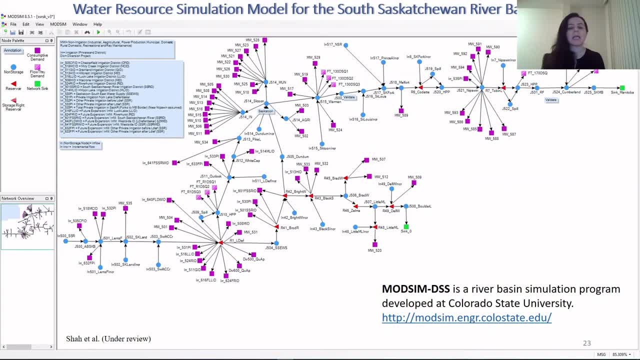 And links are careers that connect water resource or demand sites to the river basin, For example, river reaches here in this case. Now let's take a closer look at different elements of this model. here, These blue circles represent inflow. So, recalling from the structure of the model that we discussed earlier, 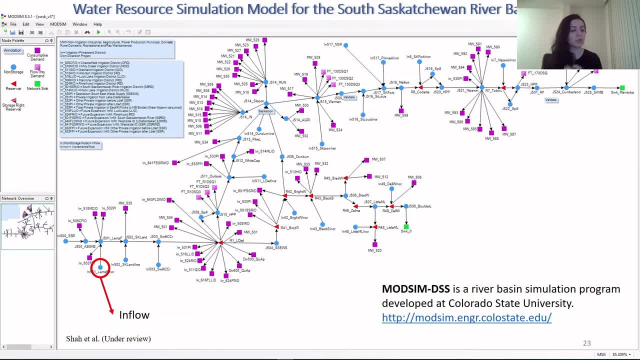 we need to enter an inflow time series for these inflow nodes here to the system Also, there are multiple nodes, purple squares here, which represent demands, And these demands are either irrigation or non-irrigation demands. And again back to the structure of the model, we need to enter time. 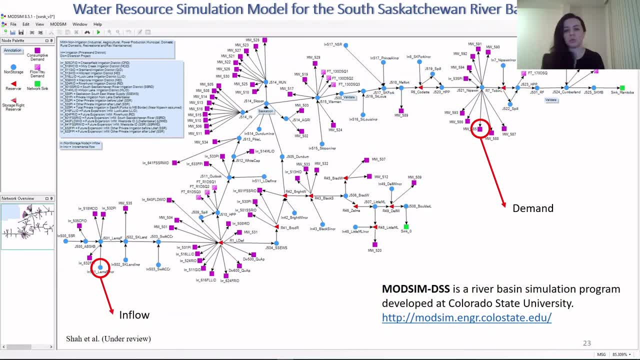 series for demands for each of these demand nodes for the model, And also you can see a tiny red triangles here that represent reservoirs, And for these reservoirs we need to define and introduce their designing characteristics, like their capacities, in the model, And also we need to 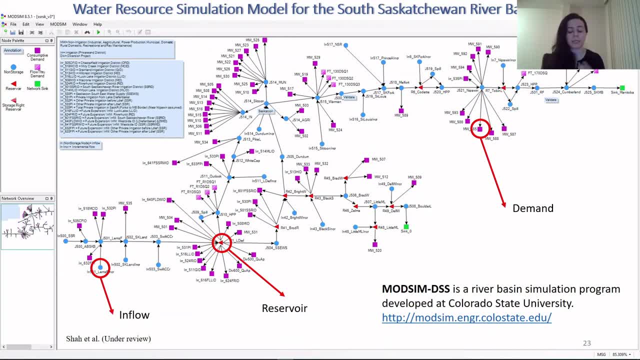 define the operating policies of these reservoirs to the model. There is another thing that we need to define here, which is the allocation water allocation policy, And here the priorities of different demands in receiving water is known And there is a licensing system that determines these priorities in place in reality in the Saskatchewan. 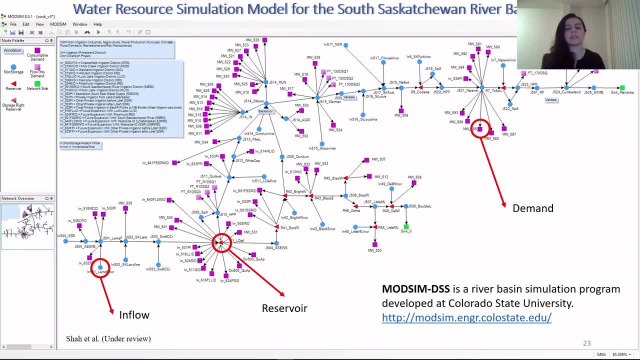 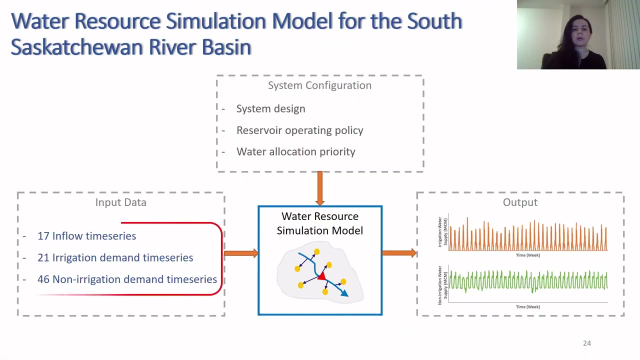 River Basin. So we used the same penalty system that I described while explaining the mathematical modeling exercise. So we also used water allocation process, чистings, also known as FIDL, to determine the bed assembled. waterранOOM Westminster 해도 noو. in this presentation to assign these priorities to different demands. in this model Now, based on what I just said, we need to provide 17 inflow time series as input data, 20 irrigation demand time series and 46 non-irrigation demands. 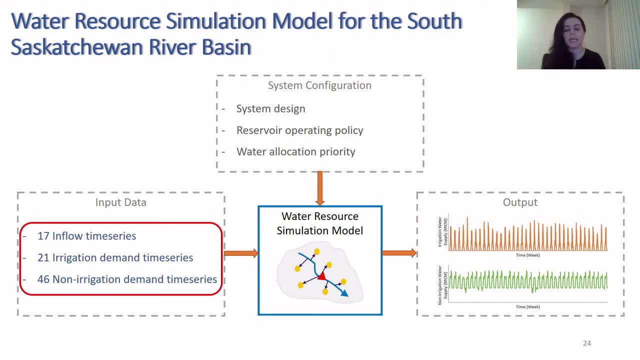 time series. So these are input data for our model. Also, we define system configurations and then we ran the model to generate outputs, And outputs here are water supply and shortages for irrigation and non-irrigation demands across the South Saskatchewan River Basin. So first we run the 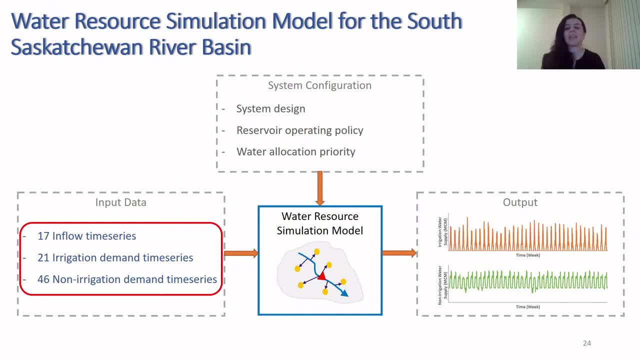 model under the status quo, before having any changes in the system. So no changes. The system is defined and configurations and input data are associated with the existing situation in the river basin, And then we are going to update the model and define a scenario. 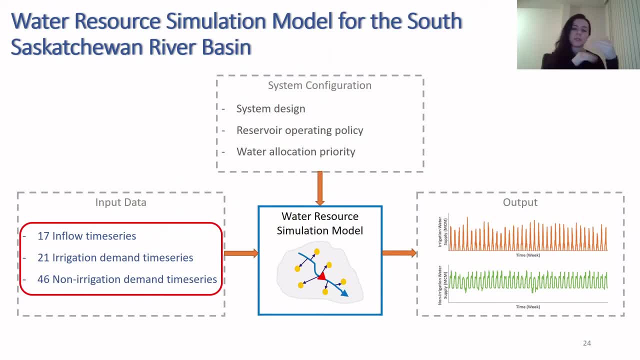 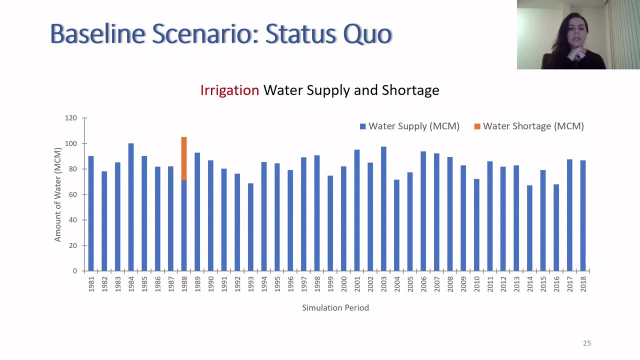 And then run the model under that scenario and then compare the results to see what would be the impact of that scenario on the performance of this water resource system. Now, under the status quo, let's take a look at the output of the model. Here are the results for water supply: 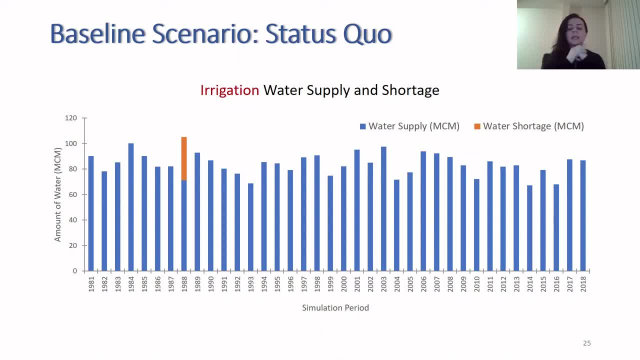 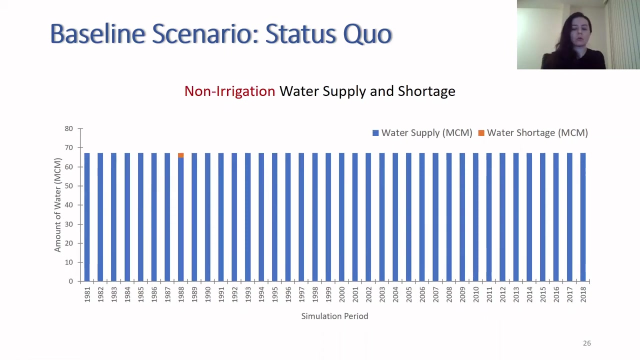 to irrigation demands. This is the total irrigation water supply and shortage across the South Saskatchewan sub-basin. Water shortages are shown in orange and, as you can see, during the simulation period, only once the water system failed to supply the total requirements for water for irrigation. Also, having a look at the water supply and shortage for non-irrigation: 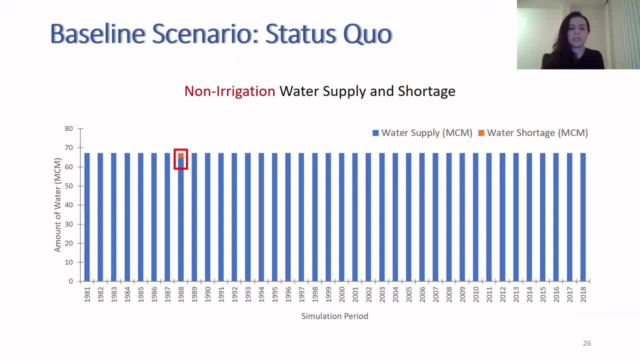 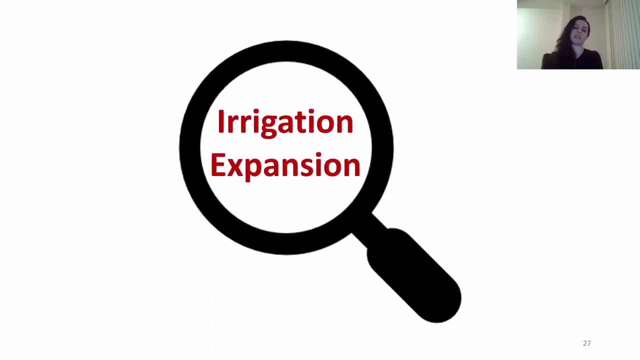 demands. we can see the same pattern here. So we only see one failure from supplying the whole water requirements for non-irrigation demands as well under the status quo. So we are now looking at the results before having any changes in the system. Now let's define a scenario and let it be. 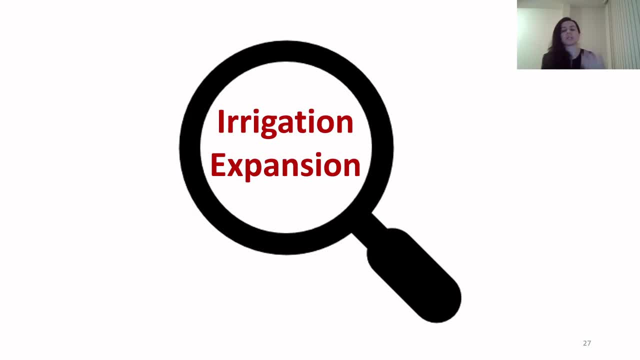 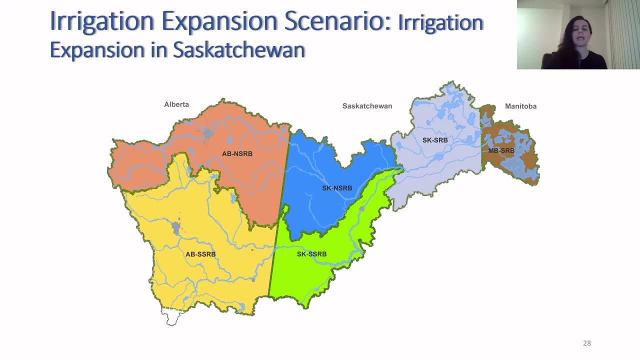 an irrigation expansion scenario How this irrigation expansion affects the performance of the South Saskatchewan river system in supplying water to irrigation and non-irrigation demands. First, a little about this irrigation expansion scenario. So this is an expansion project that is announced by the government of Saskatchewan to irrigate 460,000. 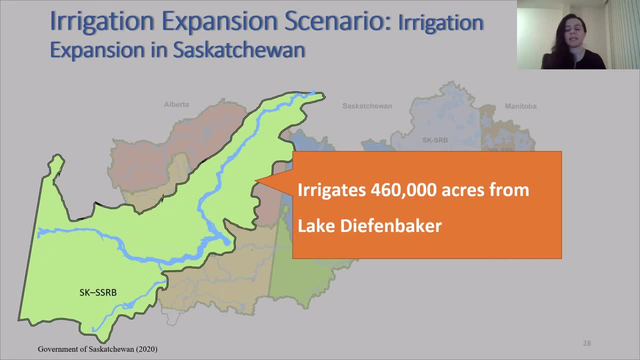 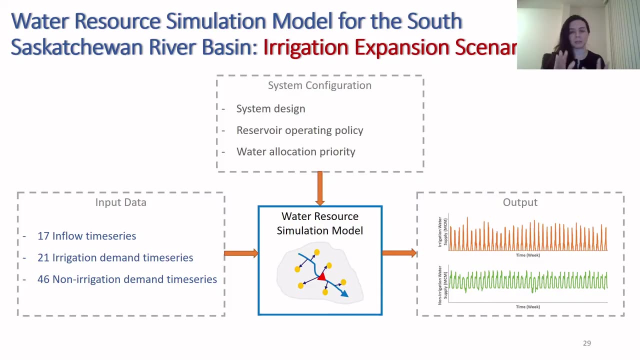 acres of irrigable lands from Lake Diffenbaker, which is the largest reservoir in this river basin, And because this scenario is sort of a socio-economic development scenario, we need to change the demand time series and update the demand time series. For that we estimate the. 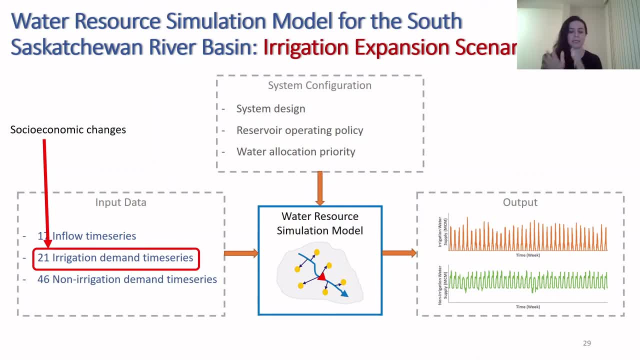 irrigation and water demand for this newly irrigated area and then add that demand as a new irrigation demand node to the system, to the model, and update the model and then run the model for this scenario under these new conditions. Now, if we compare the results- the supply and shortage for non-irrigation and irrigation- 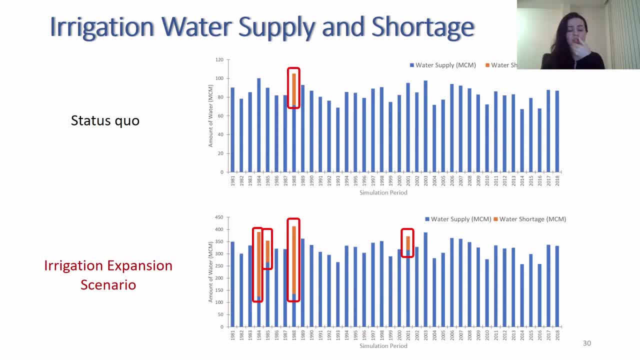 usages. here we can see that under the status code on the top of this slide, irrigation and water supply was successful almost all around the simulation period. Only once the South Saskatchewan river failed to supply water to irrigation demands, Whereas the situation that we have inして. 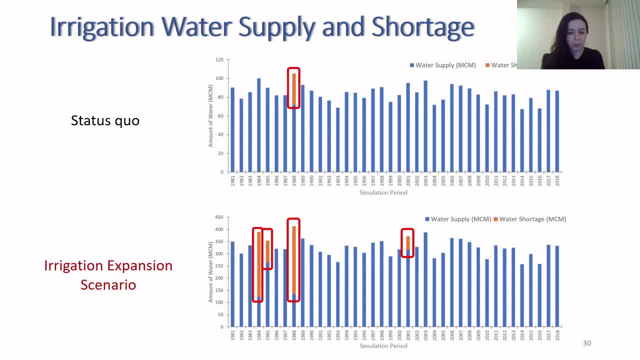 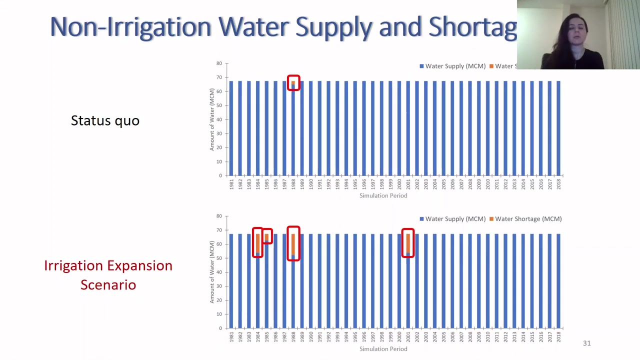 under the irrigation expansion scenario shown at the bottom of this slide, several occasions of shortage can be seen. So you can see that four times here irrigation water supply is less than water demand, so we have shortage. those orange columns- Almost the same pattern can be seen when we look at the results. 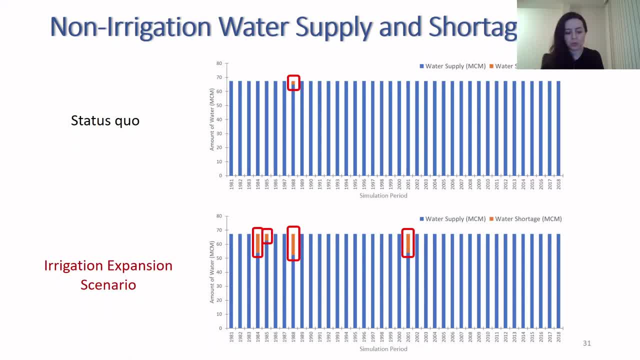 for non-irrigation, water supply and shortages. So here again, under the status quo and without any expansion irrigation. we only had one small shortage in one year during the simulation period, As can be seen at the bottom of the slide under the irrigation expansion scenario: four times the. 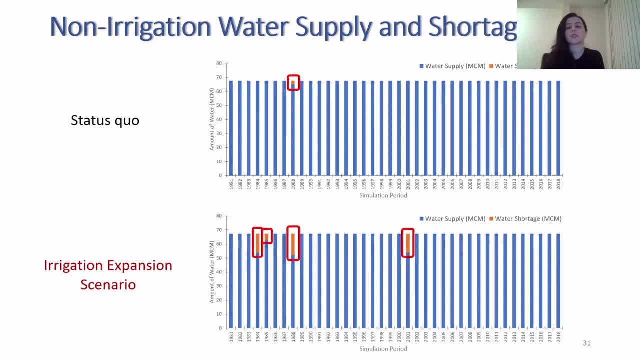 South Saskatchewan river system fails to supply and to fulfill the entire water requirement for non-irrigation demands in this river basin. So here we showed that, how we can use these water system simulation models to compare the performance of the water system under some certain scenarios, with the status quo which shows the situations without. 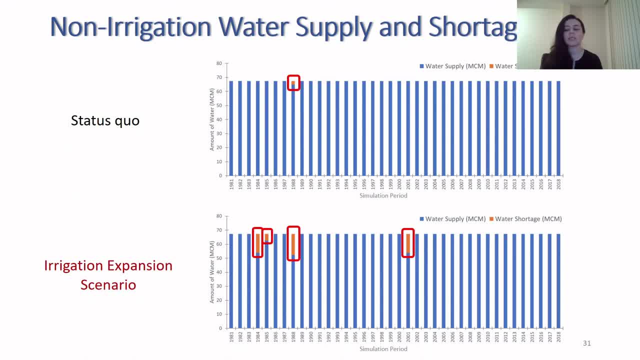 any changes in the system. This way we can evaluate the consequences of any changes that can happen in the water system to the river system and then decide to manage or to plan for our water resources. With this, I would like to wrap up this lecture. 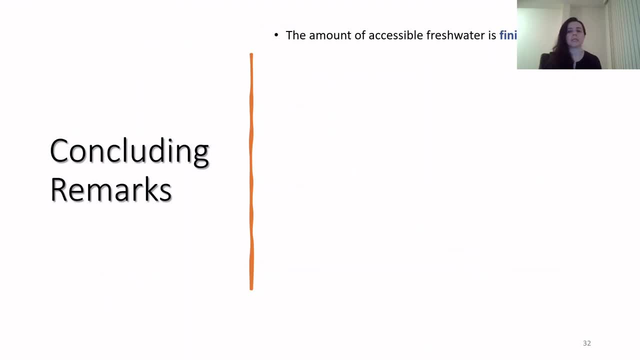 So we need to know and remember always that our water resources, our freshwater resources, are finite, which means that there is a limit to the amount of water that we can extract from these resources, and also there is a limit to the amount of pollutants that we 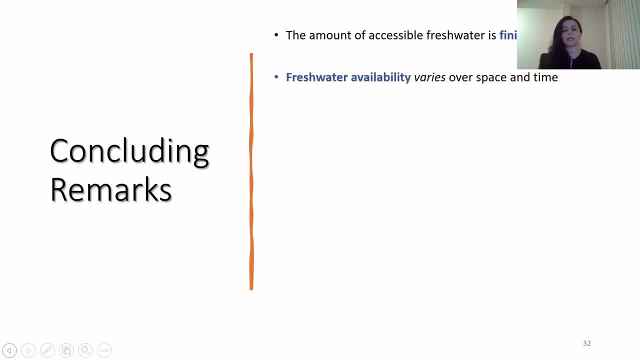 can discharge into them. Additionally, the availability of our freshwater is not evenly distributed across time and space, So we need water resource management to find effective and efficient strategies under increasing demand for water and varying supply, without provoking conflicts among users with different interests.